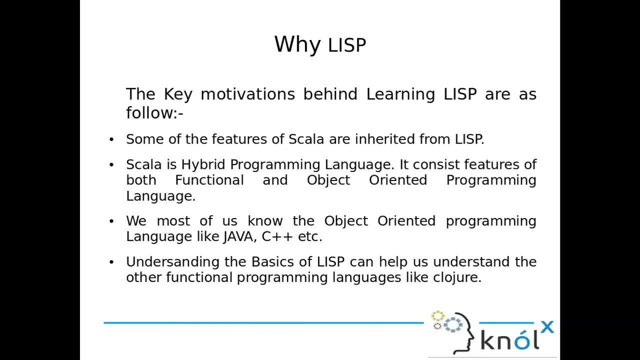 So one of the major motivation is that some of the feature of Scala are either directly or indirectly are inherited from the Lisp. If you follow the official documentation of the Scala, you will find the Lisp has been mentioned many times there because of this. And the second is, as we all know, Scala is hybrid programming language. 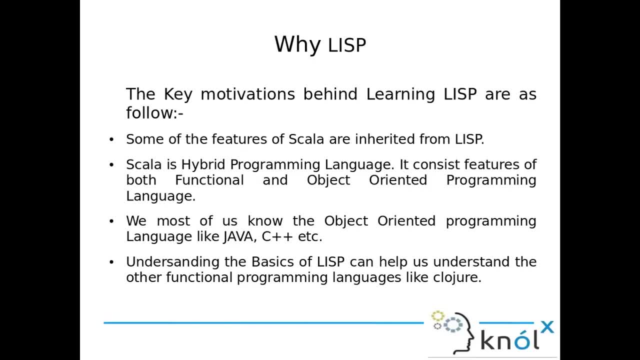 It actually consists of both features, of both functional and object oriented programming language. So from the object oriented programming point of view, We all know Java, C++ or any other object oriented language, But from the functional programming language, Scala is the first one for us. 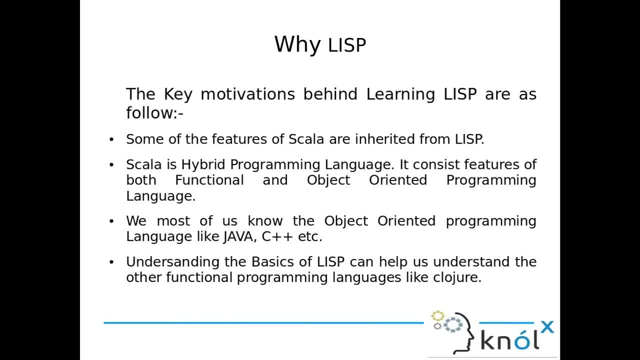 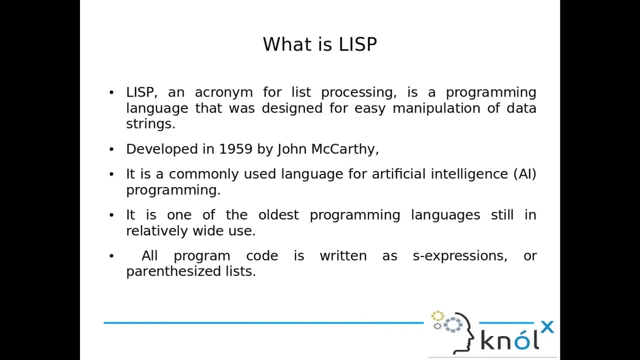 And the understanding, the basic, of the Lisp also can help us understand the other functional programming language like Closer. It is actually quite proper nowadays. So let's continue with what is Lisp? Lisp stands for Lisp programming language, So basically it is a pure functional programming language that was designed for, firstly, easy manipulation of the data strings. 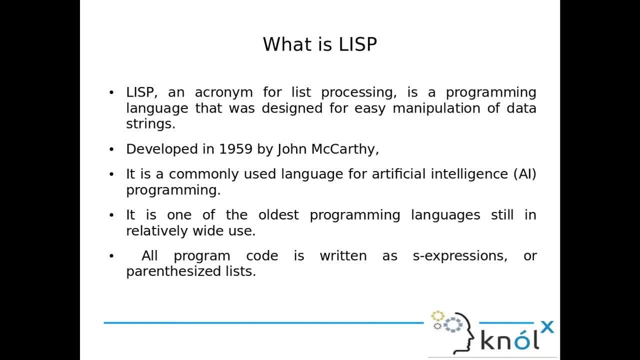 So basically, initially the major goal of Lisp is to provide the easy manipulation of the data. So Lisp is developed in 1959 and it was created by the John McCarty- John McCarty is actually the guy who tossed the gun- artificial intelligence also. 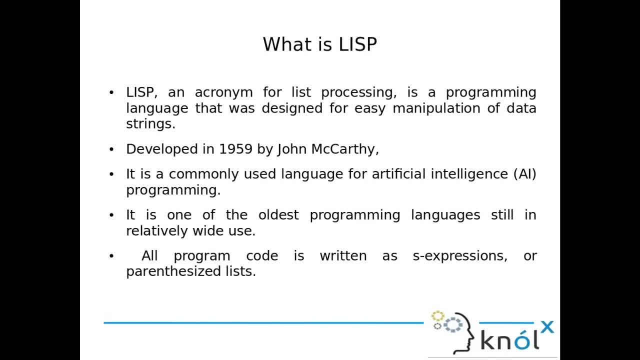 So that's why Lisp is mostly used programming language for the AI And Lisp is also the one of the oldest programming language that is still relatively widely used. And in Lisp all programming code is written as the S expression or the parenthesis Lisp, That is, each expression is defined in the parenthesis. 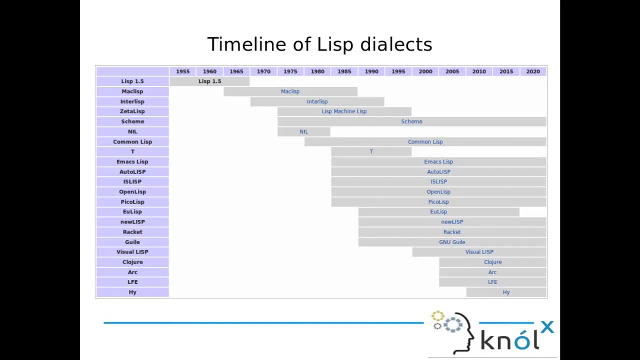 So this is how Lisp works. So this is how Lisp works. So this is the timeline of the Lisp dialect. So initially, in 1959, the first version of Lisp was released And after that many version came, like the Mac Lisp, Intel Lisp, and the one of the most common one is Schema Lisp and the Common Lisp. 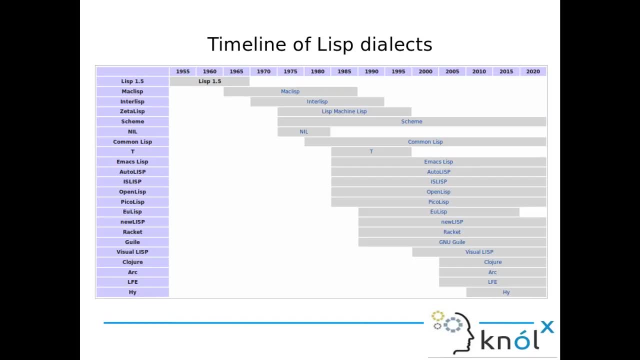 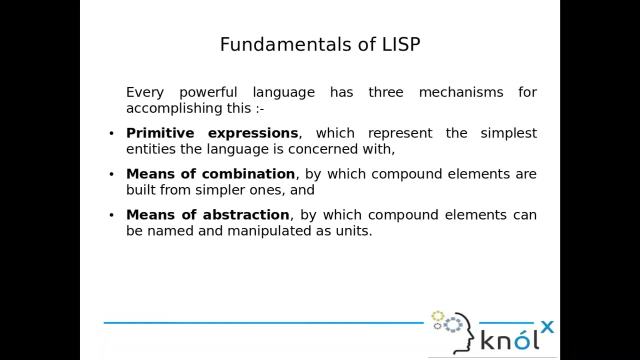 These two are the mostly used Lisp versions, And other programming language also have the base from the Lisp, like the Racket, Closer Arc and the Life. So let's quickly continue with the fundamental of the Lisp. So for every programming language there must be three mechanics for accomplishing. 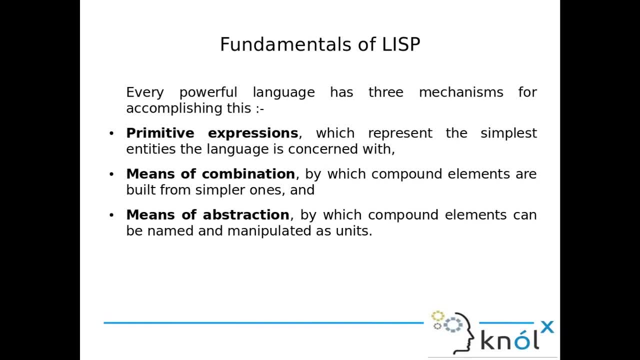 The first one is primitive expressions, So that is, which represent the simplest entity the language is concerned with, For example, a number 102, or an operator plus minus, multiplication and all. The second thing is means of combination. By which compound L? 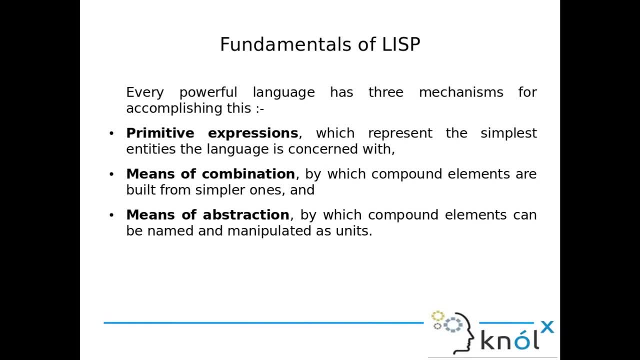 By which compound elements are built from simpler one. Compound are combination of one or more element, And elements are nothing but just a primitive expression. The last one is means of abstraction, So by which compound element can be named or manipulated as unit. So basically, in the primitive expression you can think of as the some variables. 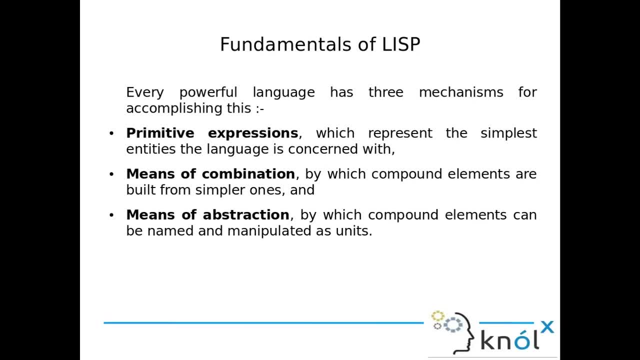 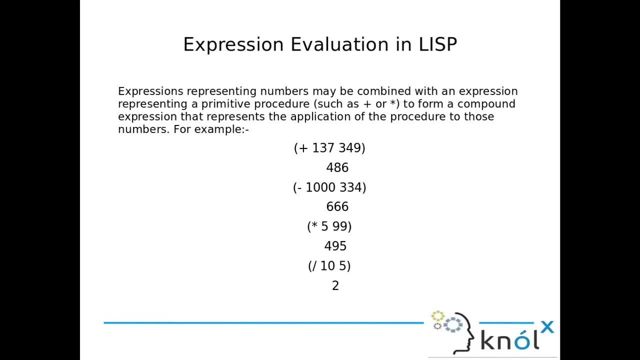 The means of combination- you can think of it as a body of the function- And means of abstraction, the naming convention in the argument of a function. You can think of this. So this is actually the simplest expression, And let's see how expression evaluation take place in Lisp. 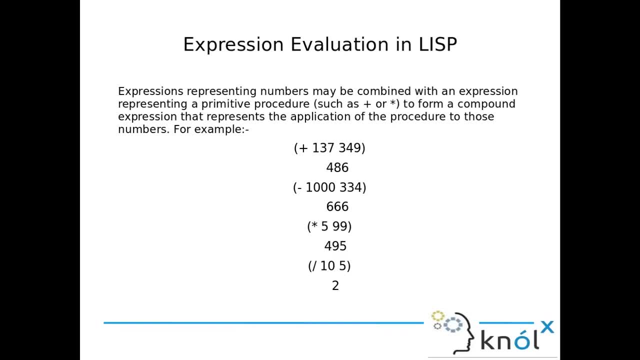 So expressions represent number That may be combined with an expression representing a primitive procedure, Such as plus, multiplication, division, and all To form a compound expression. So here compound expression is a combination of multiple expressions And that represent the application of the procedure. 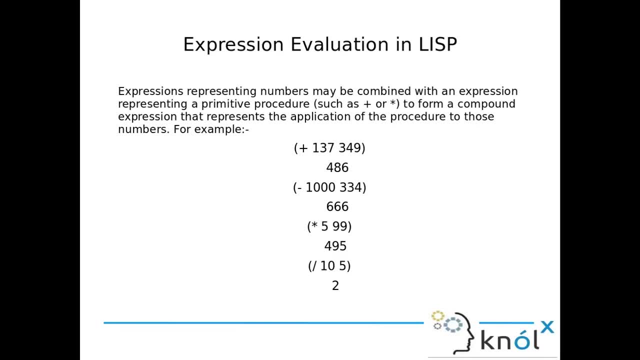 So, for example, if I want to compute the plus operator operation into the Lisp, I will start with the opening parenthesis, Follow by firstly the operator and then follow by the operand. Here you can see that opening parenthesis, then the plus operator, Then the two values 137 and 349.. 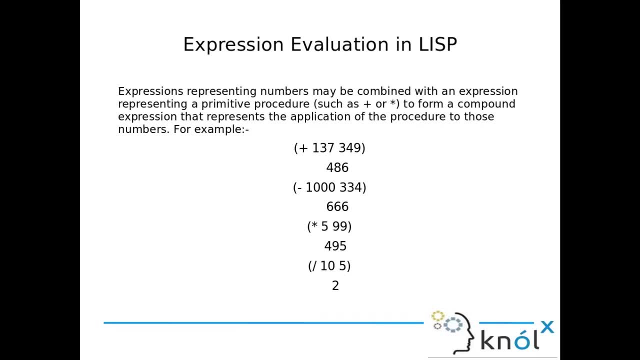 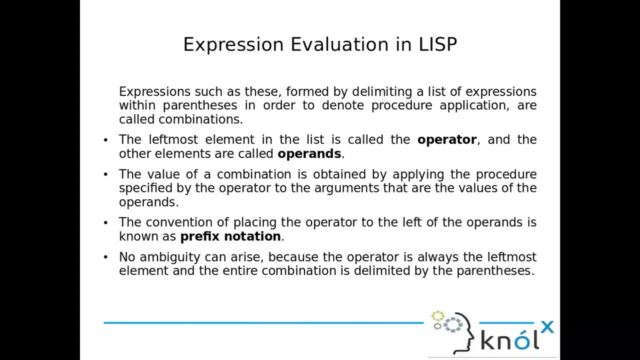 So these two values get added And the result will come as 486.. And you can see the other example of multiplication and division and all. Any question? Okay, So expressions such as these that we have seen in the previous slide Form by the delimiter, a list of expression. 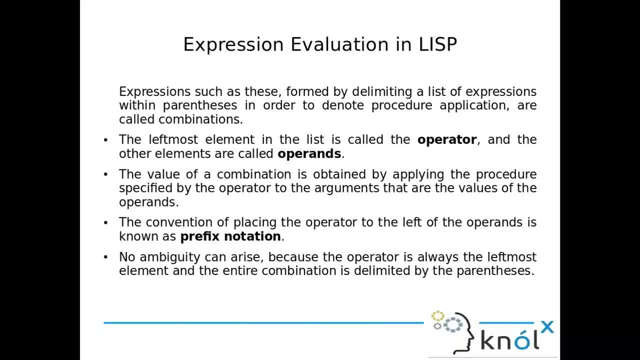 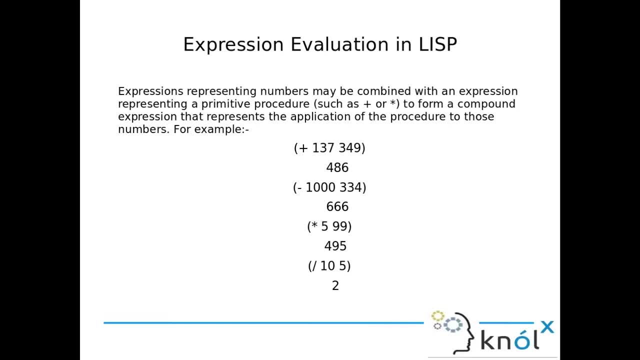 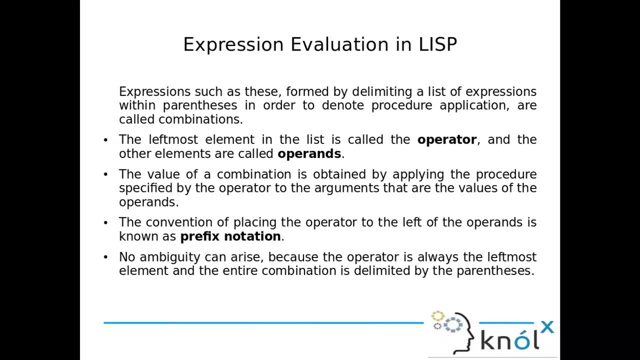 Within parenthesis, So in order to denote the procedure application, These are actually called the combinations, Because these are the combination of some values or the simplest expression. So inside the parenthesis, The left most element in the list is called the operator. What operation we need to perform? 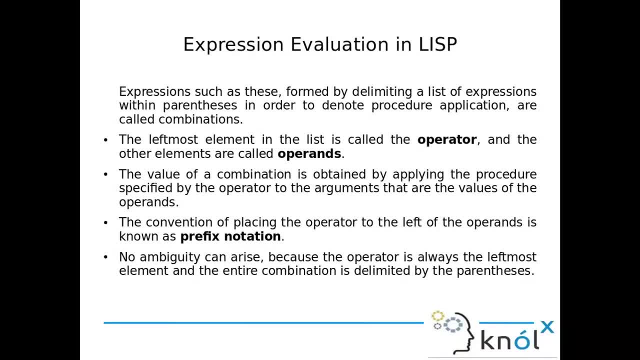 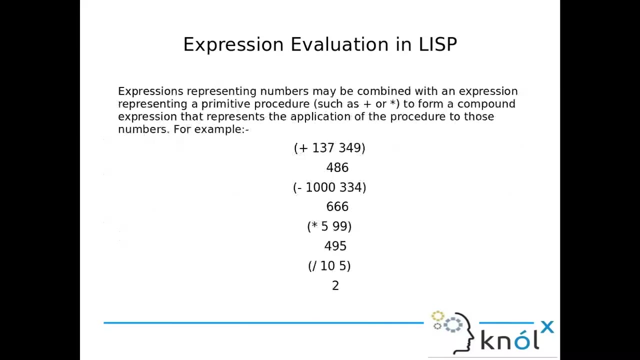 And the other element are called the operands On which we need to perform the operation. Secondly, the value of combination is obtained by applying the procedure Specified by Specified by the operator to the argument that are value to the operands. Nextly, the convention for placing the operator to the left of the operand is known as prefix notation. 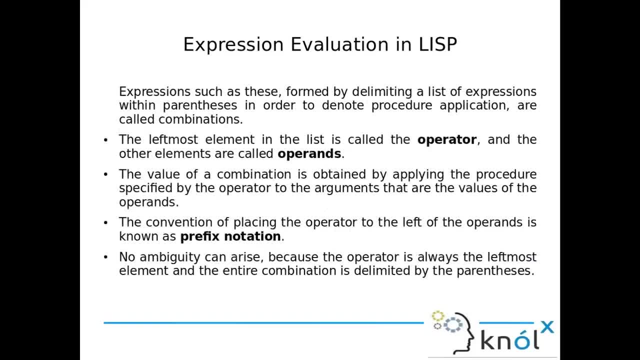 We start with the operator, then the operands. So due to this, there can never be ambiguity, Because the operator is always the left most element And the entire combination is delimited By the parenthesis. So we start with the operator, then followed by the operand. 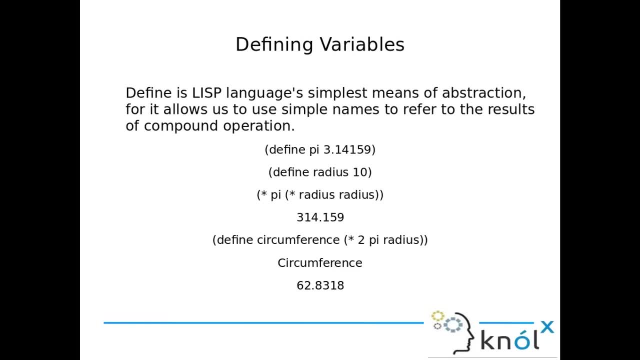 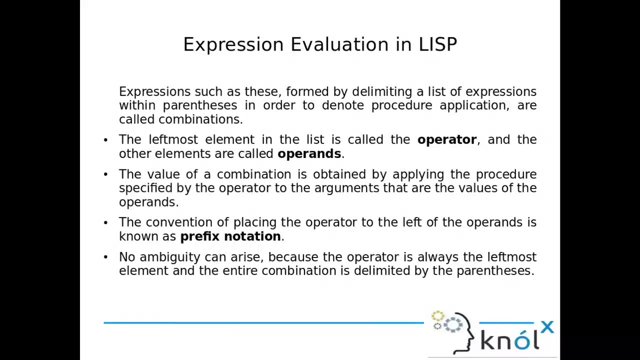 This will be the whole structure in the list: Defining variables in list. So for defining the variable in list We use the define keyword. So define in list language is the simplest means of abstraction. This is the third one means of abstraction. 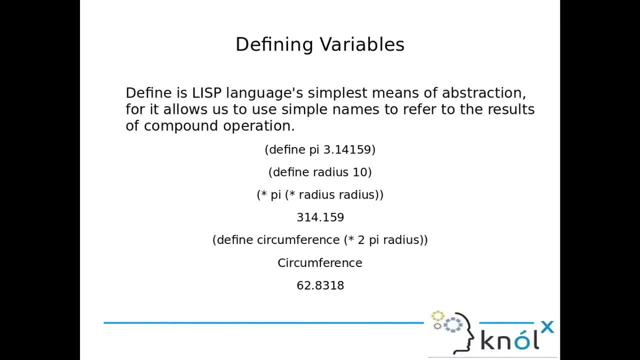 That we are following here. So for this it allow us to use simple names To refer to the result of the compound operation. Suppose, if I want to define some variable pi And giving some value, 3.14.. So what I will do is: 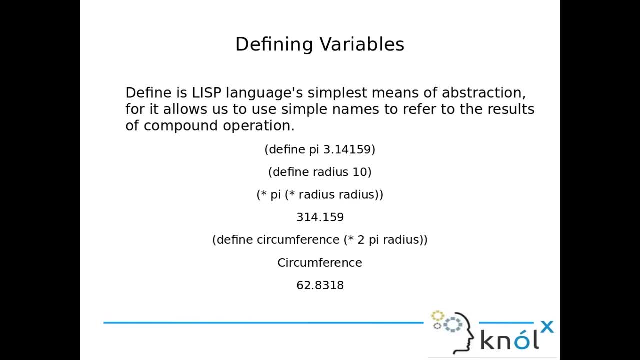 I start with the opening parenthesis, Then use the keyword define, Then after that name of the variable, And then the corresponding value, And with the closing parenthesis, And I can also compute some kind of a computation using these parenthesis, Like you can see in the third line. 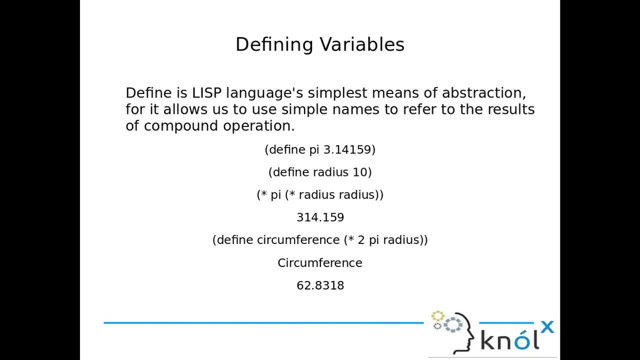 I am multiplying the value of pi. Then, furthermore, I am actually multiplying the radius by itself. So here the value of radius is 10. And the pi is 3.14. So I will get 314.159 as the output. Same goes for circumference. 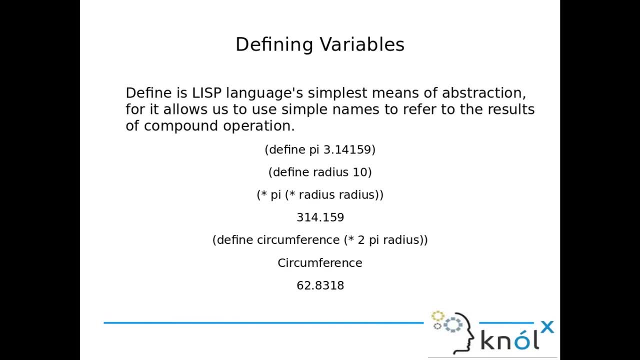 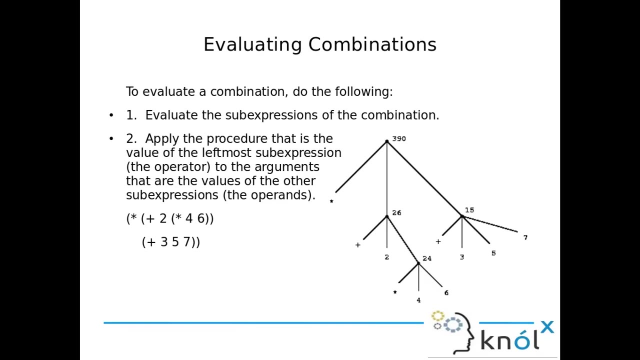 Here, circumference is a variable, Not a matter, Because we are directly assigning value. Not directly, but in form of a simple expression. So let us see how the evaluation combination- Evaluating the combination- take place inside the list. To evaluate the combination: 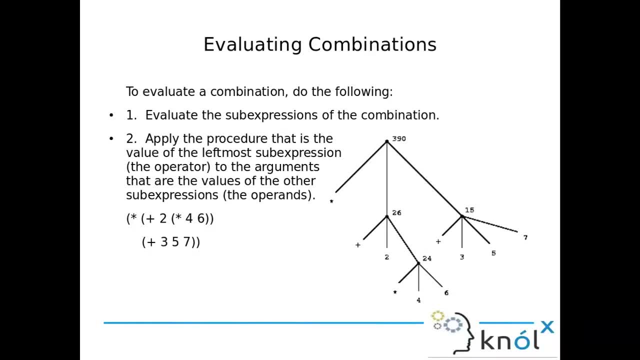 We do the following thing: Firstly, we evaluate the sub-expression of the combination And then what we do is We apply the procedure, That is the value of the leftmost sub-expression, That is called the operator, To the argument. That are the value to the operator. 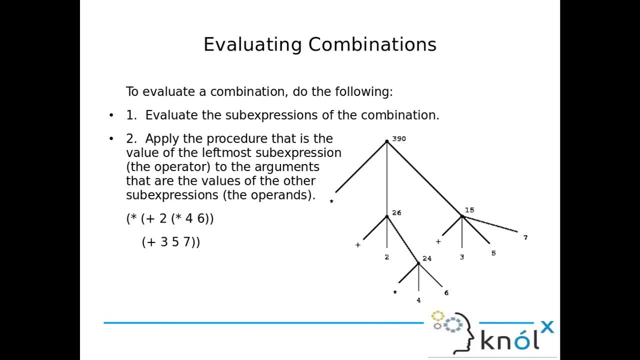 That are the value to the other expression. So let me explain this. So here we have the expression Multiply Plus 2.. Multiply 4., 6. And the next line, we have addition of 3., 5.. 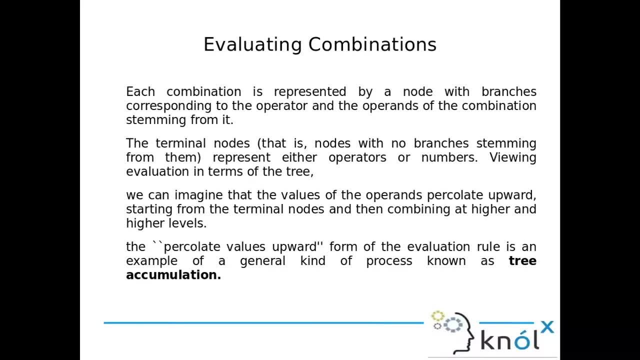 And 7.. So what will actually happen is Each combination is represented by the node, With branches corresponding to the operator and the operands Of the combination streaming. So the terminal node, That is actually the last one, Or the leaf node. 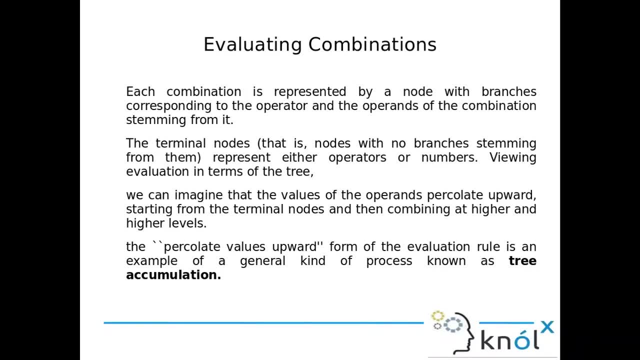 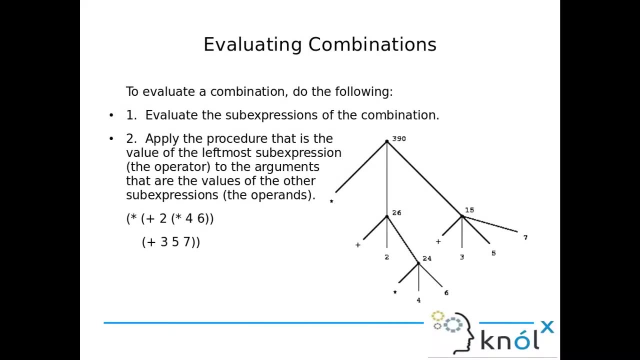 It can either represent the operator Or some numeric value. So now we can imagine that The value of the operator Generated upward, Starting from the terminal node And then combining at higher and higher level. So here you can see that The lowest level of sub-trees 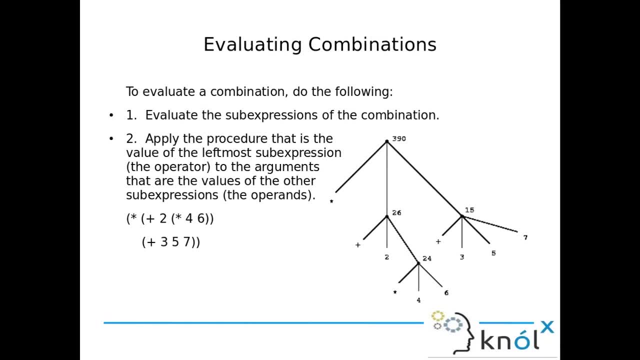 Multiplication of 4 by 6.. So firstly we will evaluate this expression That will give us The value 24.. Then this 24 will become input for the Higher level of expression That will- We will add- with the 2.. 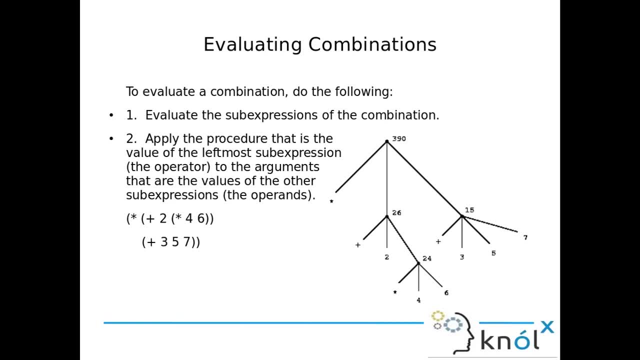 We will get 26.. Then we will perform the addition of these 3 values: 5., 3., 5. And 7. And then we will multiply The value of these 2 expressions And we will get the final output. 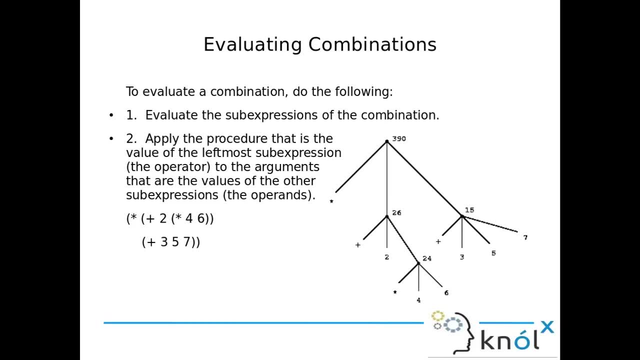 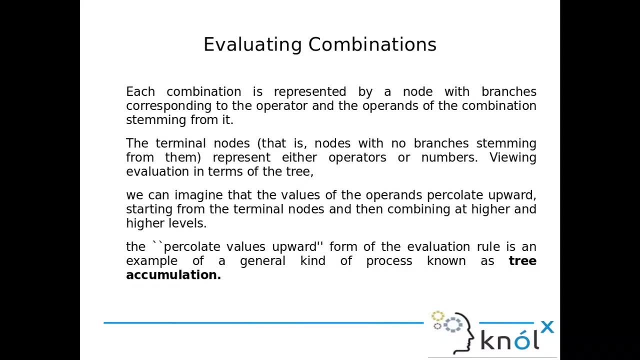 3. 9. 0.. Ok, So this generation or Perculate Values upward, Formed up In the final output: 3. 9. 0.. Ok, So this generation or Perculate Form of evaluation rule. 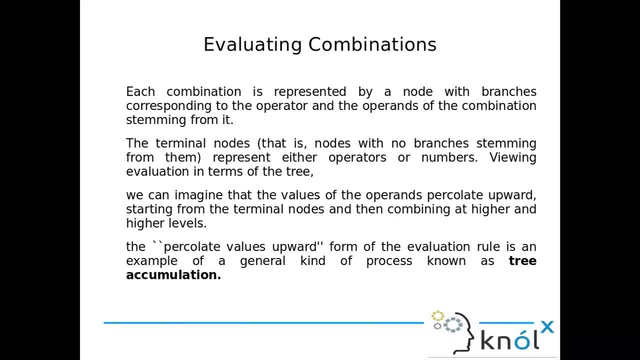 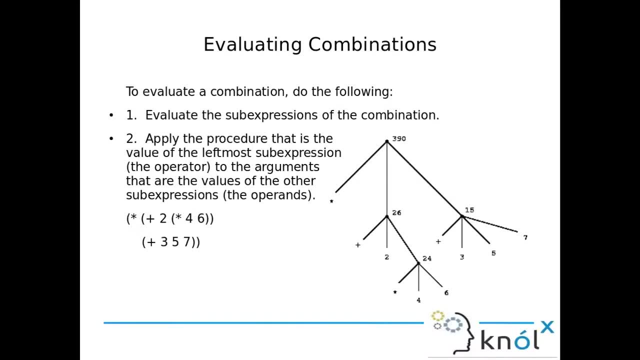 Is an example of A general kind of process That is called Tree accumulation. So basically A normal tree is generated For each expression, Then it will compute, it Start from the terminal node And then sum up to the Higher and higher level. 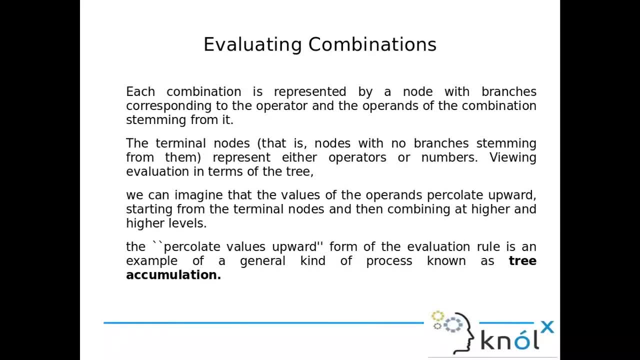 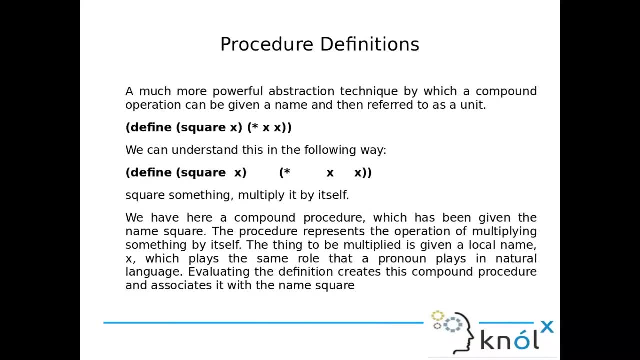 The next is Procedure definitions. This is actually the much more Powerful Abstraction technique By which A Compound operation Can be given To the Form of Evaluation Rule That is called Tree Accumulation. 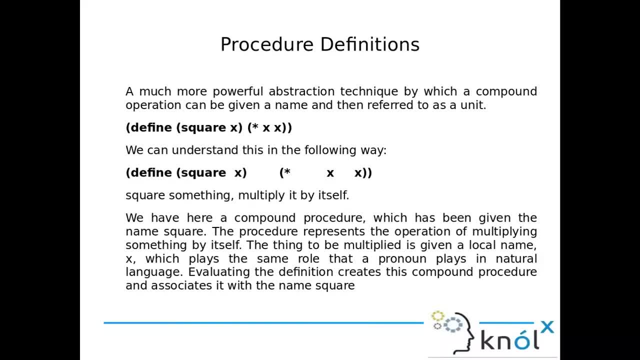 So basically, Tree Accumulation Can be Given a name Or referred to As a unit. So this is actually How we define The method Or the procedure Inside the list. So we start with the Opening parenthesis. 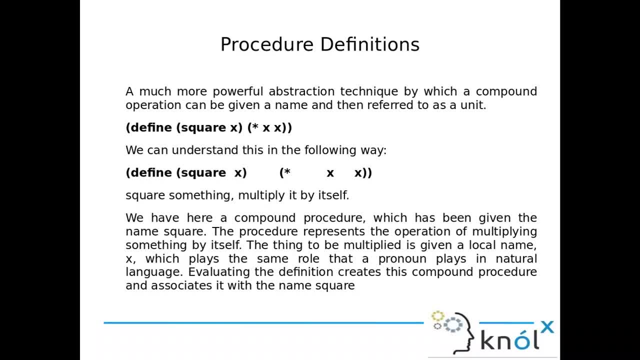 When we use the Define keyword, Then we start with the Another parenthesis, Then we give name to the Method Or the procedure Follow by the local variables Or the argument, Like here we have X, Then we give the body. 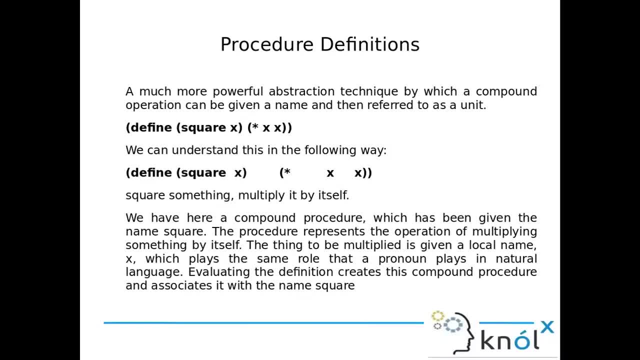 For a square, X should be Multiplied by X. So here we have A compound procedure Which has a Given the name Square, The Procedure Representing the Operation Of multiplying Something by itself And the 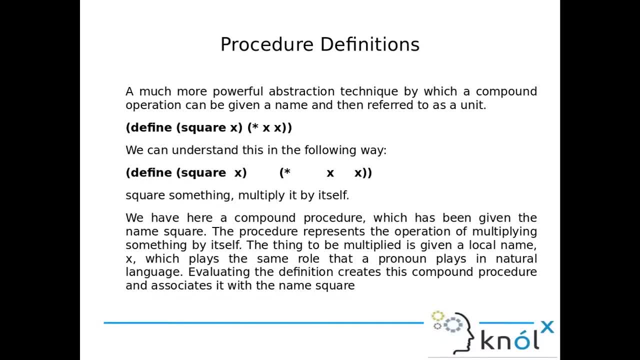 Thing of multiplying Is given by the Local name. That is X here That we use And that is pronounced In natural language. Evaluating the Definition Create this Compound operation Associates It with the Name. 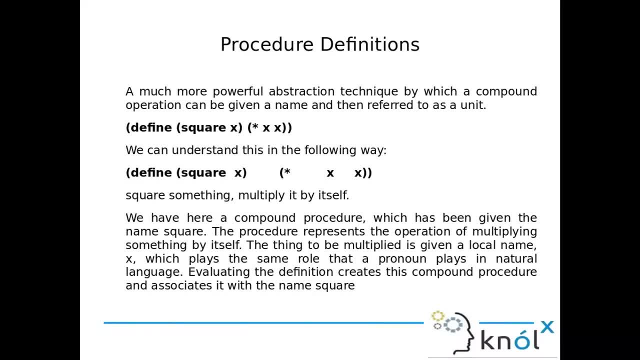 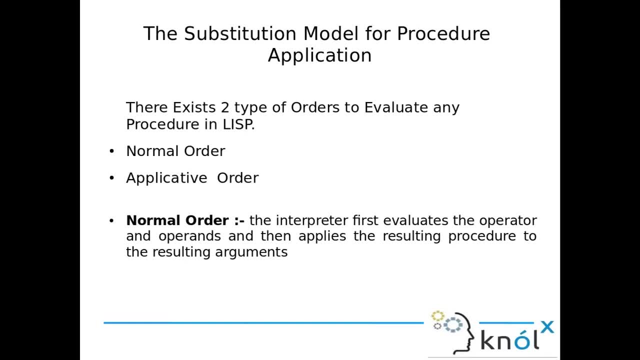 Square. So basically, Instead of Using the Square And We can Get the Corresponding Square Of that value. The next, The substitution Model For Procedure Application. So basically Expression Can be: 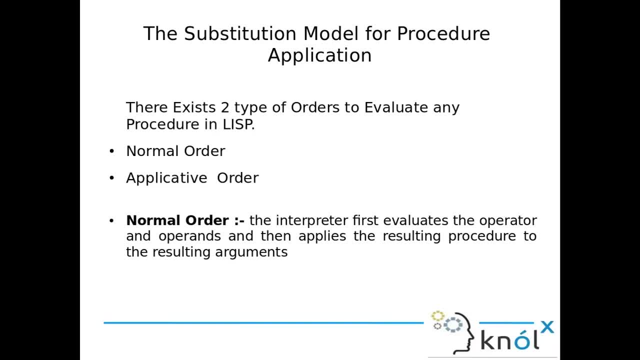 Evaluated In two ways. Firstly There is a Normal Order, Secondly There is a Applicative Order. So basically, In normal Order We can Evaluate The Square And The Operands. 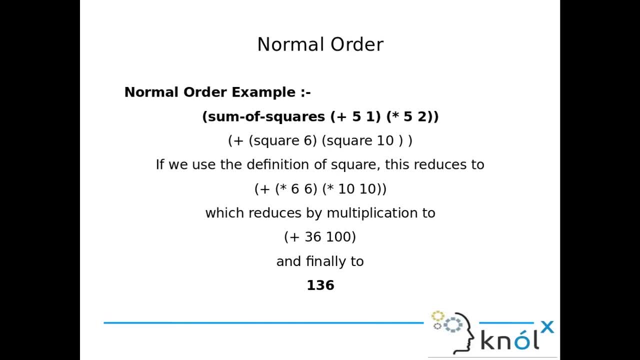 And then Applies The Resulting Procedure To The Resulting Argument. Let Me Explain This With The Help Of Example. Suppose I am Computing A Square Six. 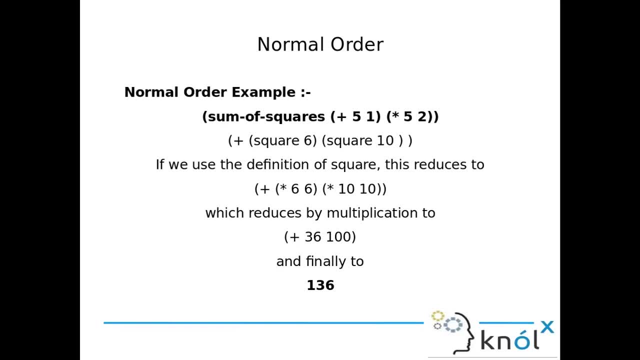 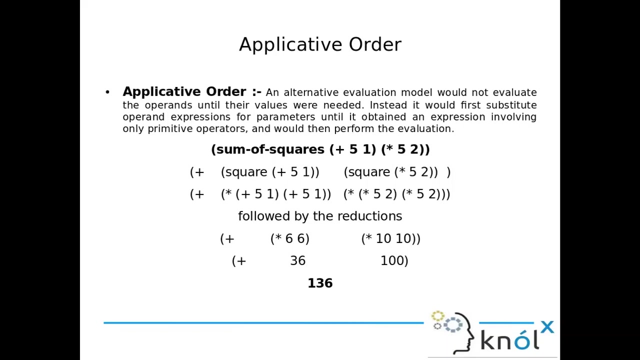 And Square Ten. Then After That I Will Give The Body Of The Square, That Is, Six Multiplied By Six, Ten Multiplied By Ten, Correspondingly. 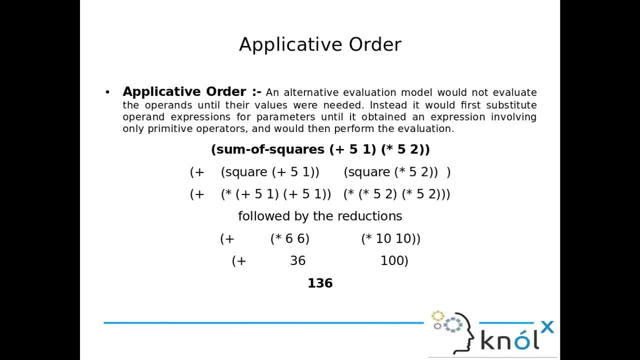 Then I Have The Result In The Expresion. So Basically In This Model, This Model Would Not Evaluate The Operand Until Their Values Are Needed. 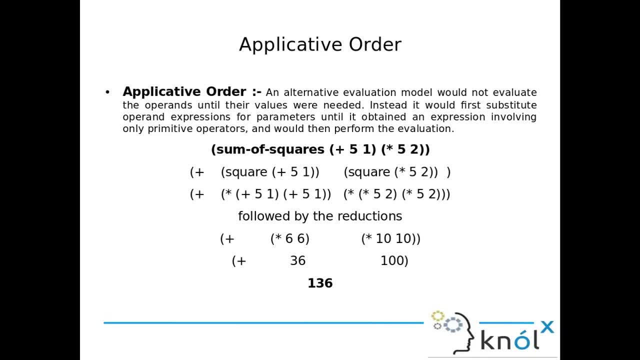 What It Will Do Is: And The Five Multiplied By Two. So Here You Can See That Instead Of Computing The Value Five Plus And 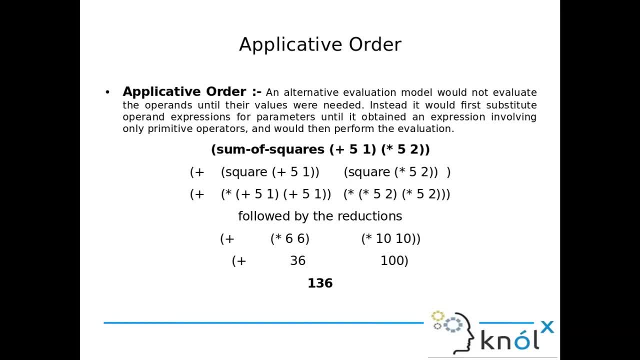 Five Multiplied By Two, We Are Actually Firstly Giving. Now We Can. We Cannot Expand This Expression Further, So That's Why We Will Continue To. 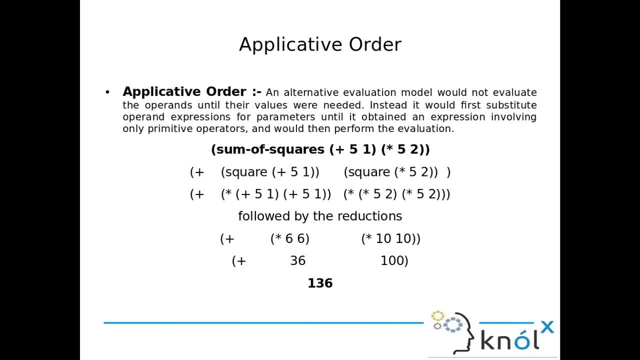 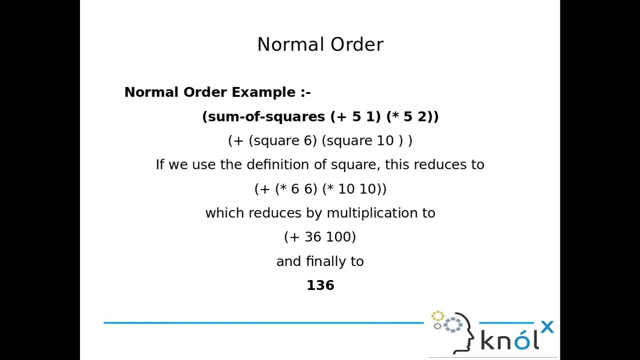 The Reduction Part. So Here You Can See That We Will Add. These Two Get Manipulated Twice By The Interpreter, So That's Why It Is. 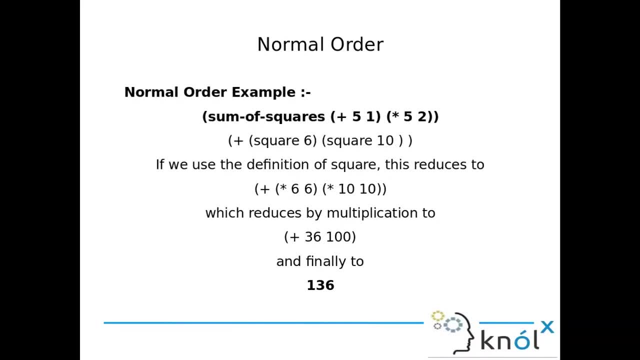 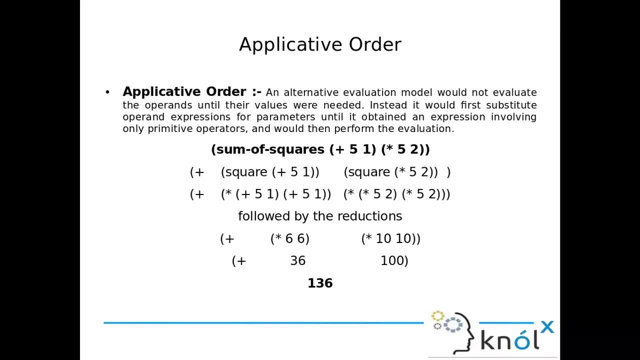 Not Optimized As The Normal Order. So That's When Actually By Default Is Actually Takes The Normal Schema, I Think, Yes, There Is A Normal. 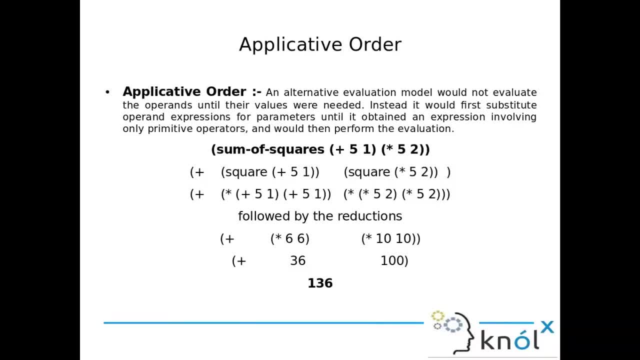 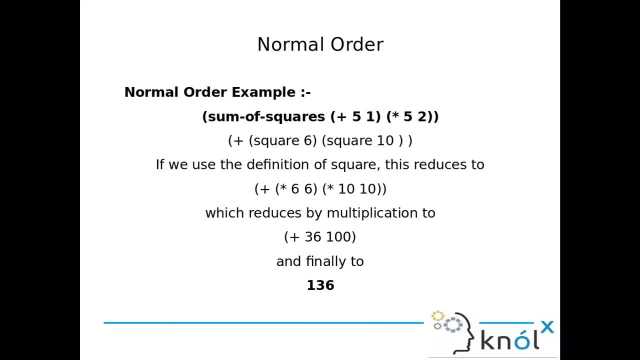 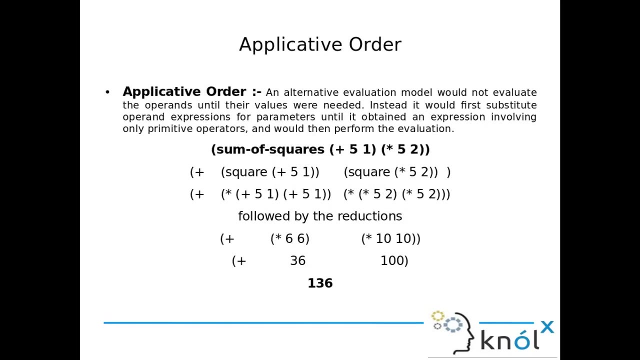 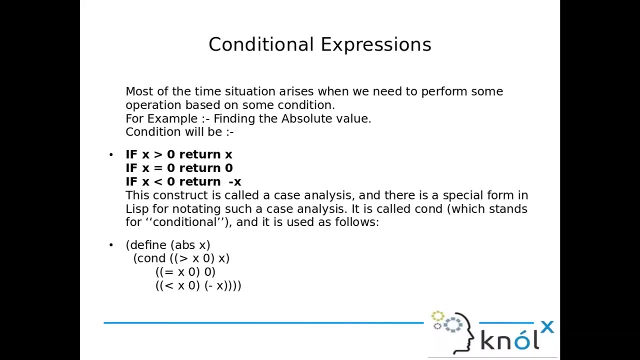 Order, But I Think, Into The Common, We Can Change It To The Applicative Order Also. Yes, That's Why The Default Order. Okay, The Next. 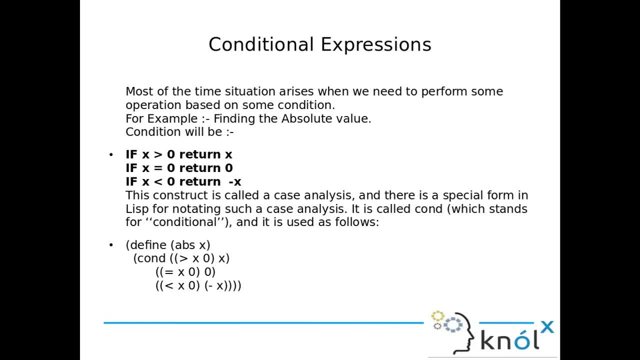 One Is The Conditional Expression. So, Basically, What Will Happen? Most Of The Time The Situation Arises When We Need To See The First One. 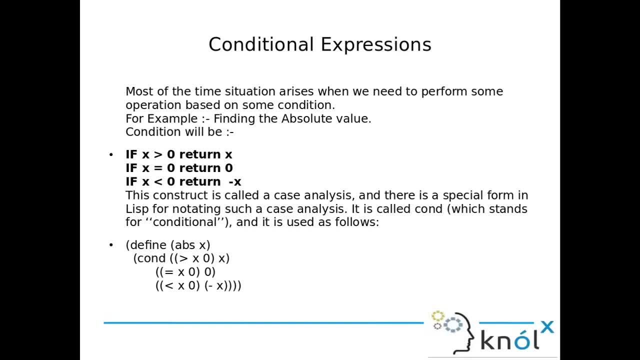 Is: If X Is Greater Than Zero, Then Directly Return The X. If X Is Equal To Zero, Then Return Zero, And If X Is. 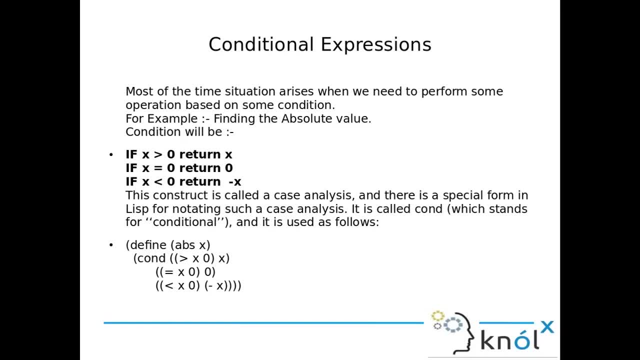 Greater Than X Zero, Then There Is A Special Form Of List To Notate Such Case Analysis With The Help Of Keyword: Conditional, So What. 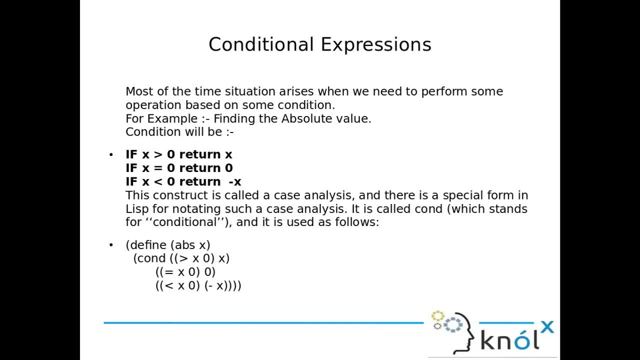 Actually Happen Is This Case: We Will Return X. The Second Is: X Is Equal To Zero. In This Case, We Will Return The Zero. 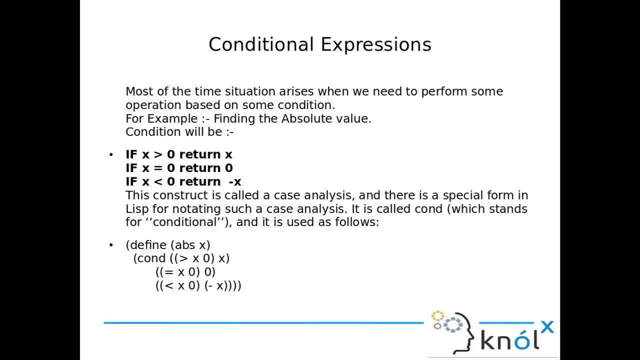 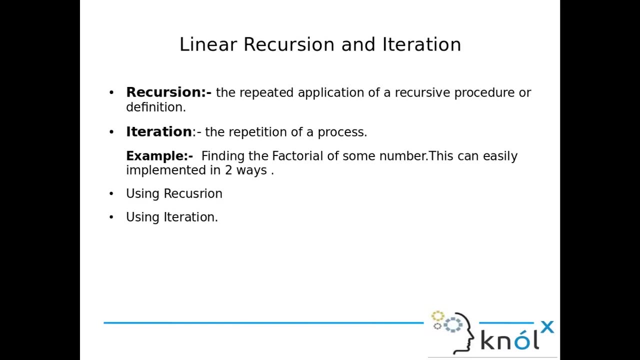 And In The Last Case That Is X And This Is Also So. That Is Why In The Minus X We Are Using The Parenthesis. 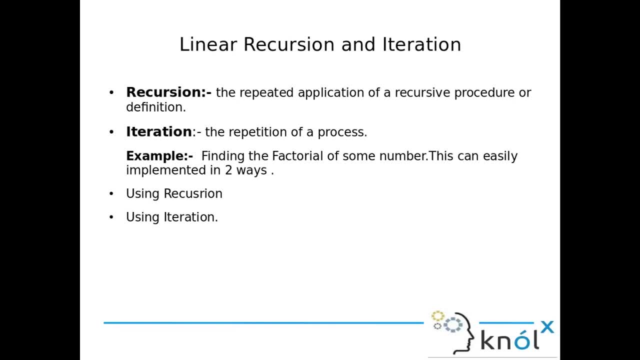 Also. So This Is Actually The Quite Popular One. The Major Difference Between The Result At The End, Right An Iteration, Is Strictly Similar To. 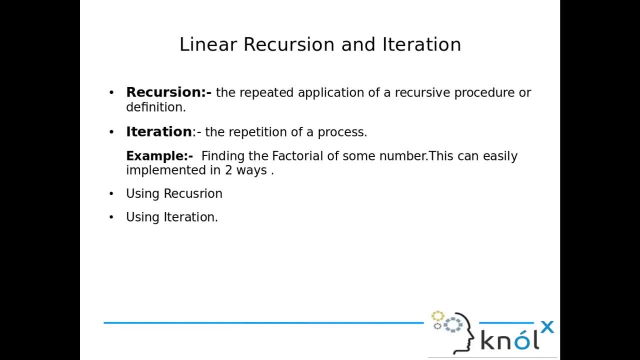 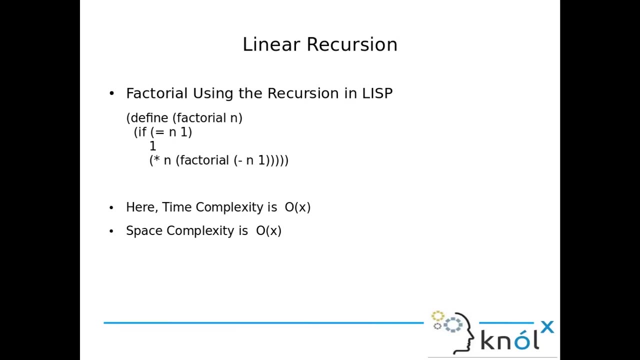 Recursion, But The Condition Varies According To The Iteration. So Let's Take An Example, So That We Have The Factorial Using The Recursion. 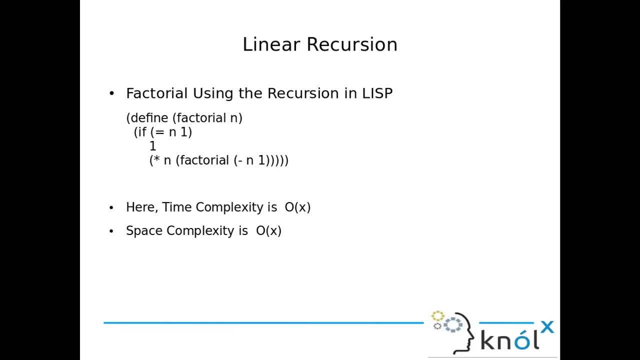 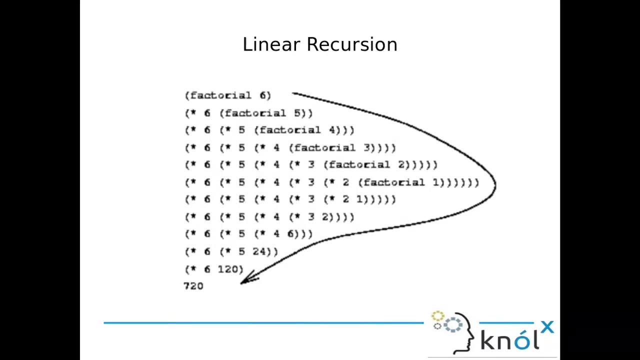 In List. So Basically, What We Have Done Is We Have Defined The Method Factorial. This Is Actually Using The Recursion. So If We Start, 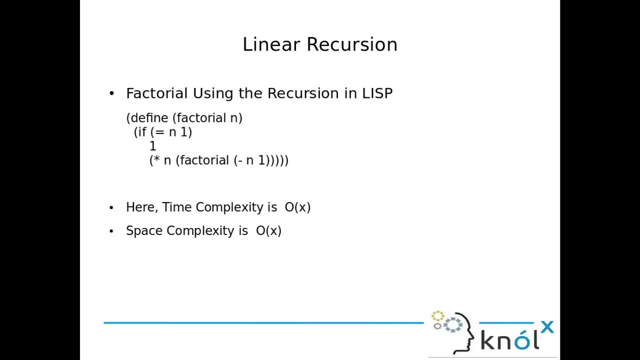 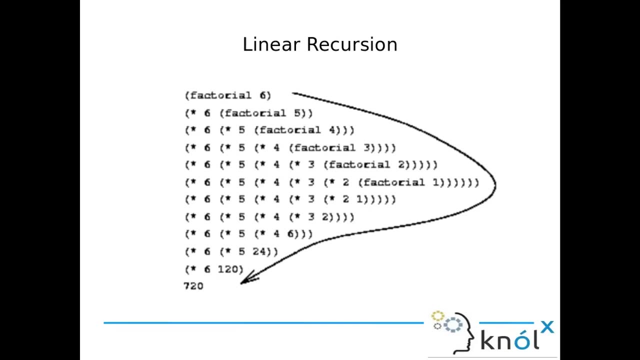 With The Factorial Of Six, Then What We Will Do Is It Will Go To The Second Condition, That Is, Multiply The N By Factorial. 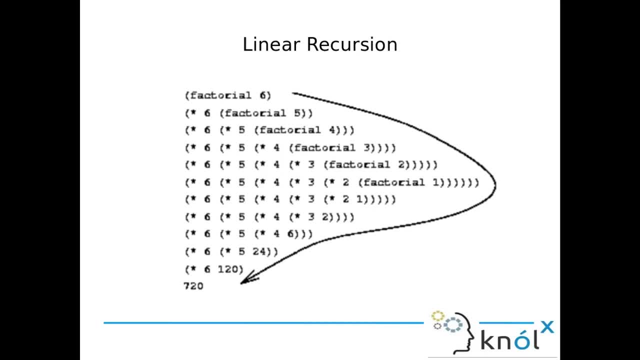 Of N-1.. We Will Start Computing Or Manipulating The Expression. So Firstly The Multiplication Between Two And One Take Place, Then The Corresponding 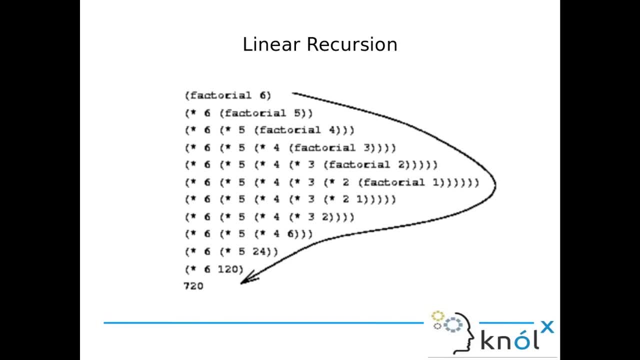 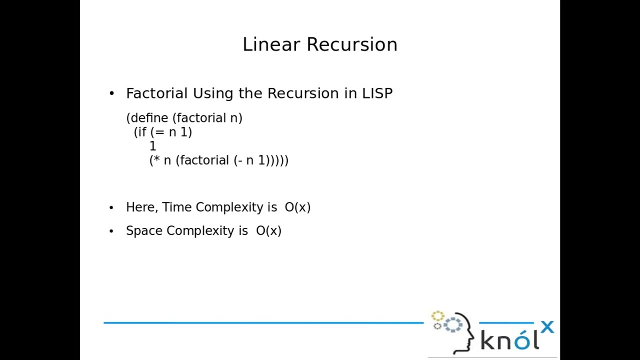 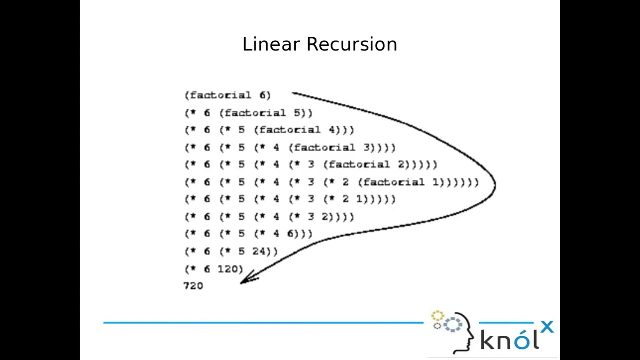 Result Will Multiply By Three And The Corresponding, So Basically The Time Taken By This Method Or The In The Linear Recursion Will Equal To 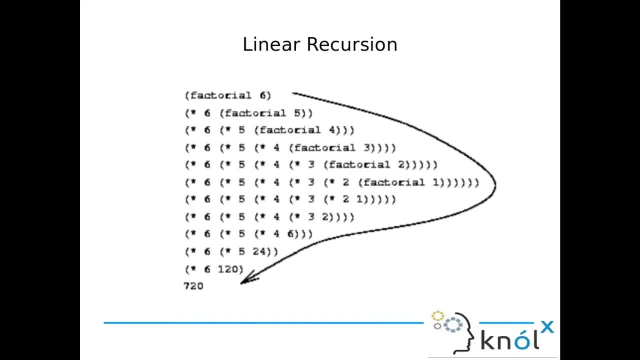 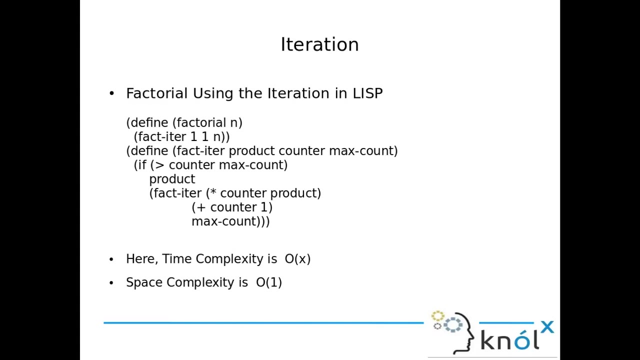 The Big O Of N Or The Big O Of X, Whatever. The Second One Is Factorial, Using The Iteration In List. So This Is: 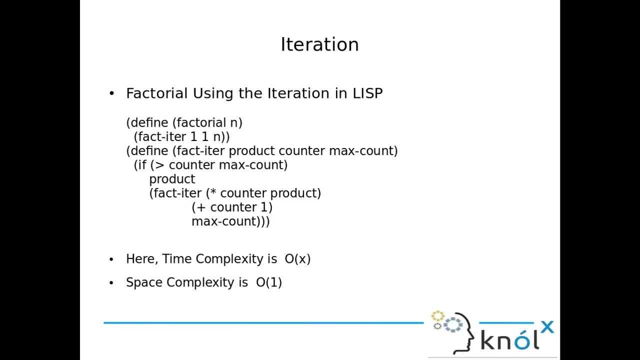 Actually Slightly Confusing. So Here We Have A Function And The Nested Function. So Firstly, We Just Know Our Cover, Current, Current Stage Of The. 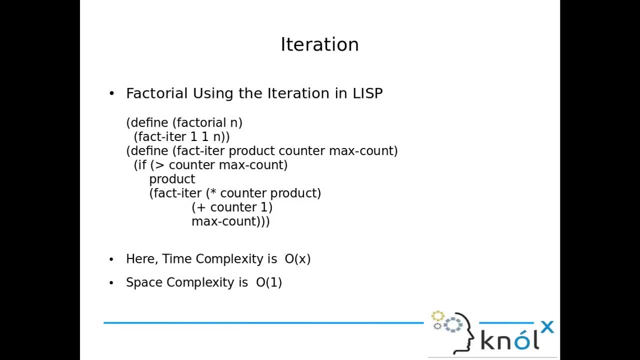 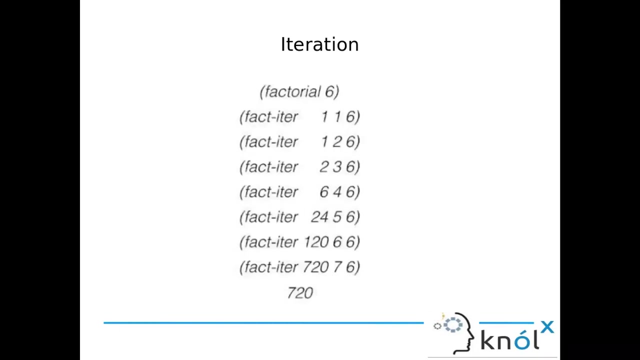 Counter, And The Maximum Count Will Restrict Us To Exit From The Loop. So Basically, The First Condition Is If We Have One, So Here, 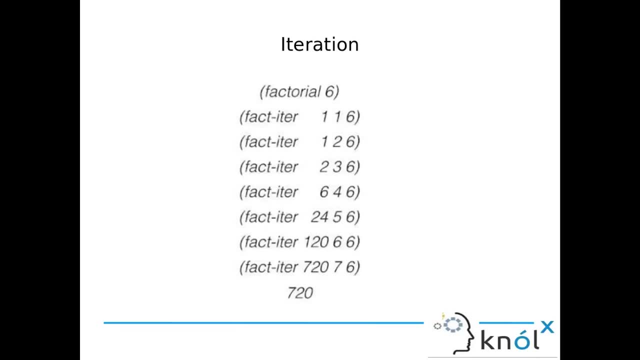 You Can See This In The First Iteration: The Value Is One One Six Product Is One, Counter Is One, Max Count Is Six In. 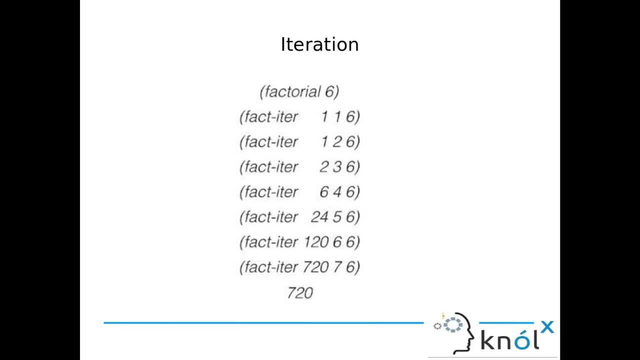 The Next One. We Will Multiply The Product And The Counter That Is Equal To That Will Give Us One. Multiply By Two That Is Equal. 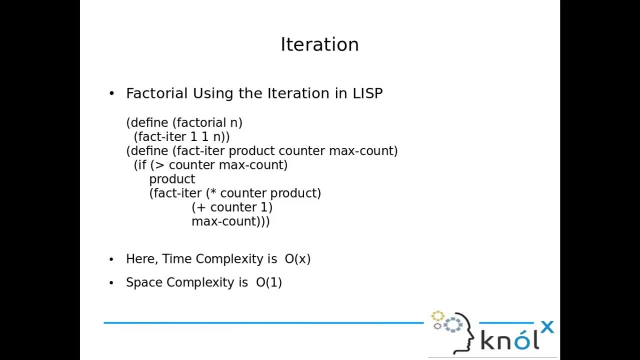 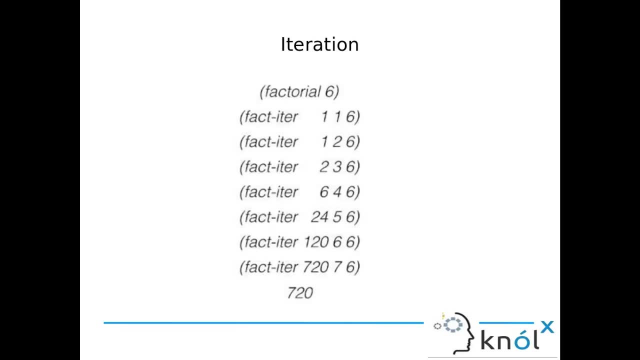 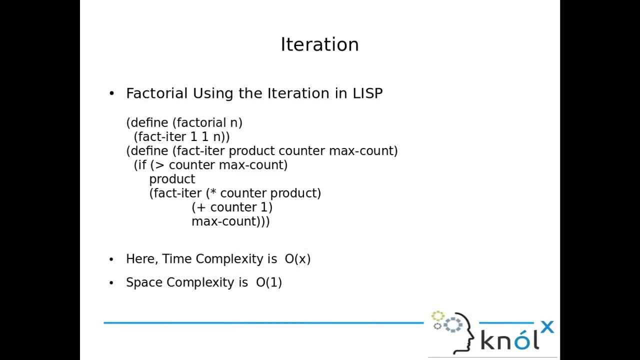 To Two. One Is One Is Equal To The Big Of X Because It Is Still Taking. Whatever Input Is, Has Been Given That Amount Of. 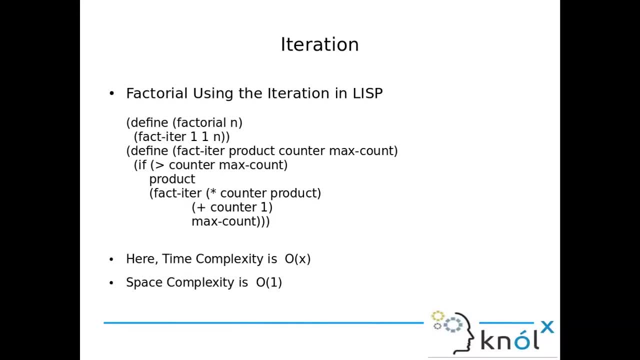 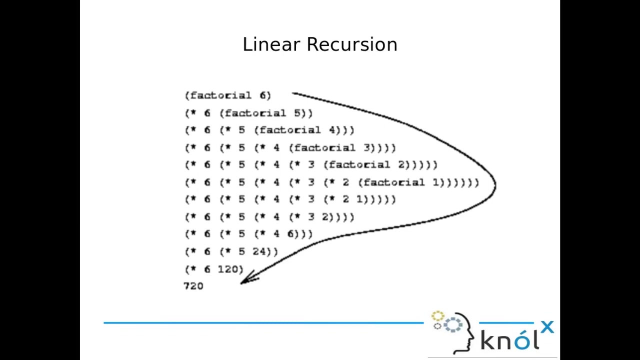 Time For Computing Each Value. No, It Is Yes After The In Scala, After The Internal Implementation, Because It Will Convert Into The Value Inside. Yes, 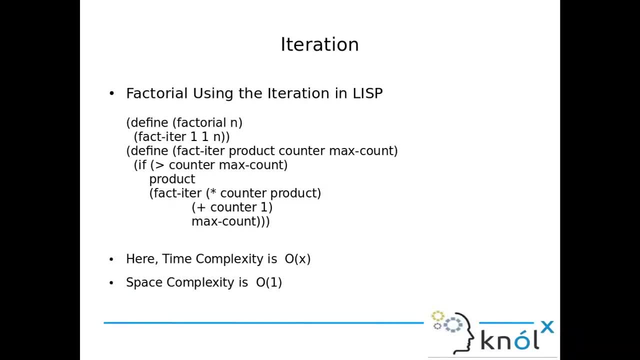 Yes, The Issue That We Are Faced With I Will Cover Up Into The Next Knowledge. Actually, It Will Yes, Yes, Yes, Yes, Yes, Yes. 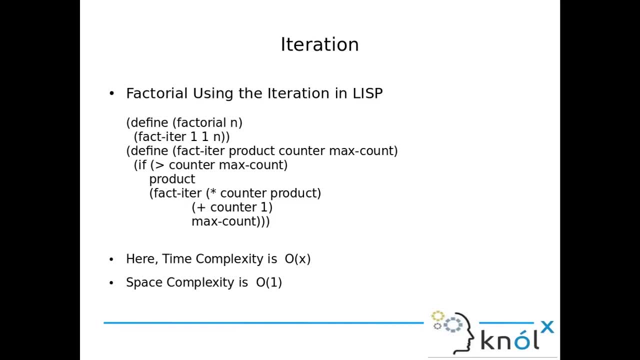 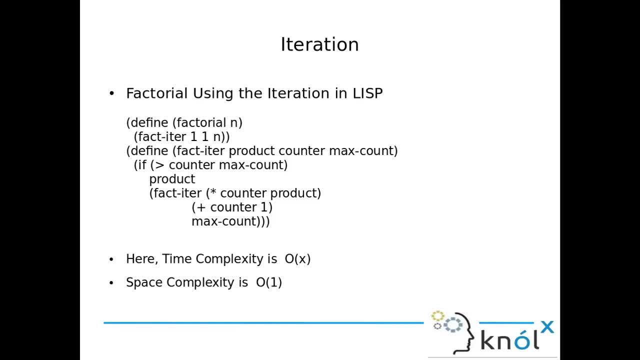 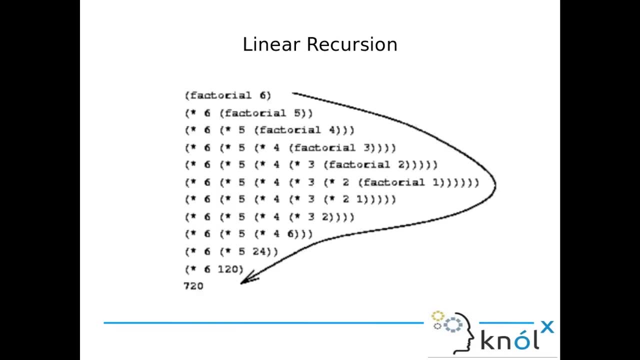 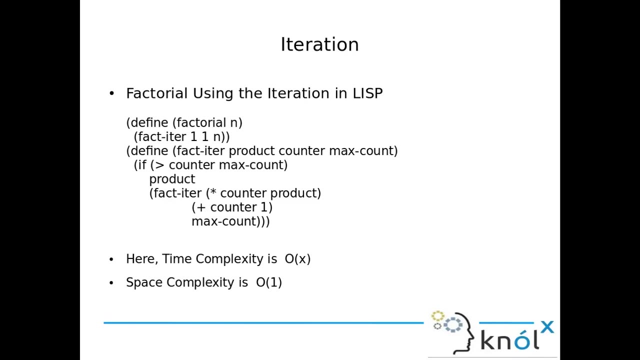 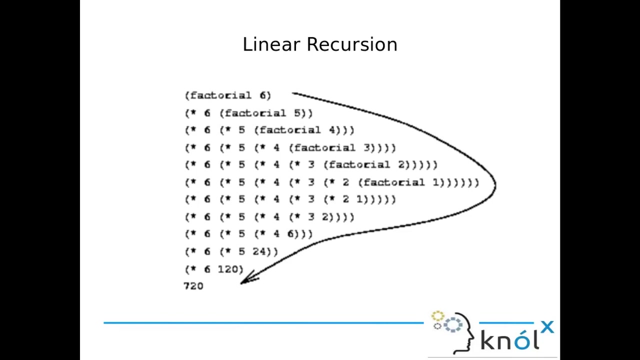 Minor Difference You Can See Here. I Am Calling The Directly Function Fact Writer Here And Yes, yes, it will After the if memory get linear. yeah, inside the iteration. 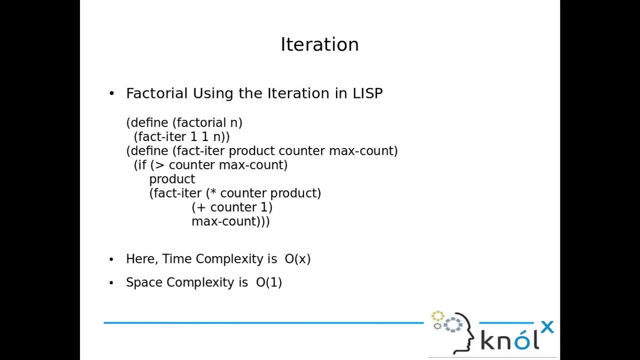 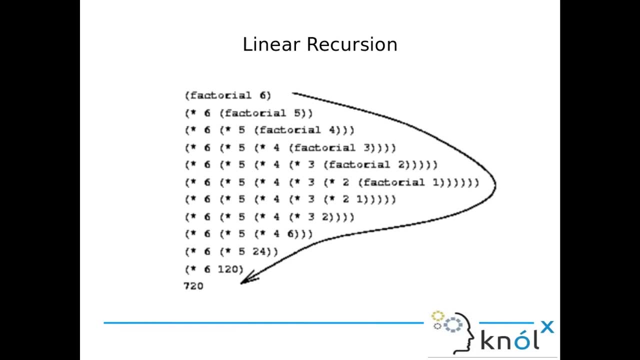 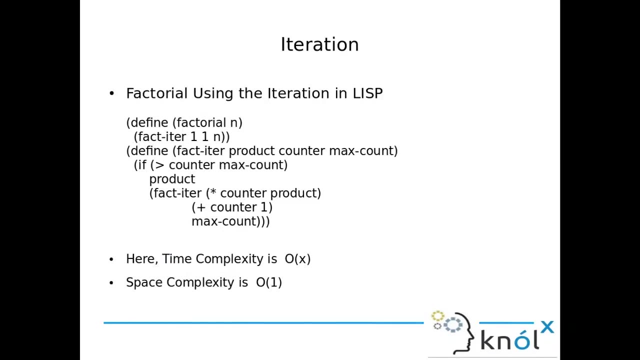 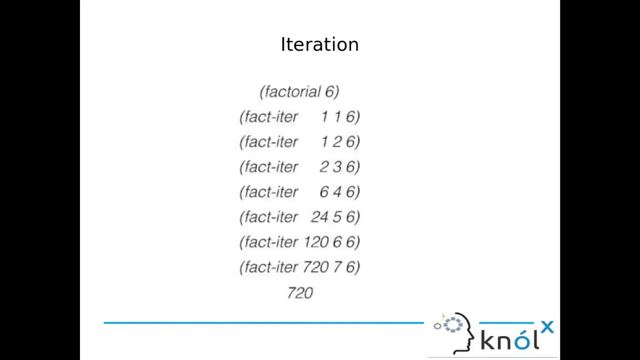 Yes, in that case that will directly convert it into the iteration one Iteration. That's why we use the annotation at tail rack, just to notify. So this is all the. these are all the fundamentals of the list. So any other questions? 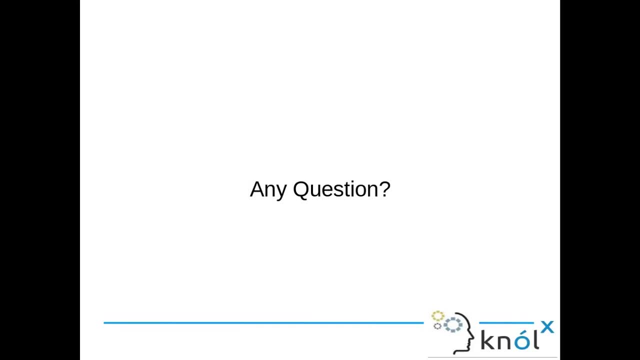 So basically, in the next knowledge I will cover the much more advanced methods that are high order function inside the list. So basically, in Scala we can either take function as high order function as argument or can return In return. what we can do is we can use the both. 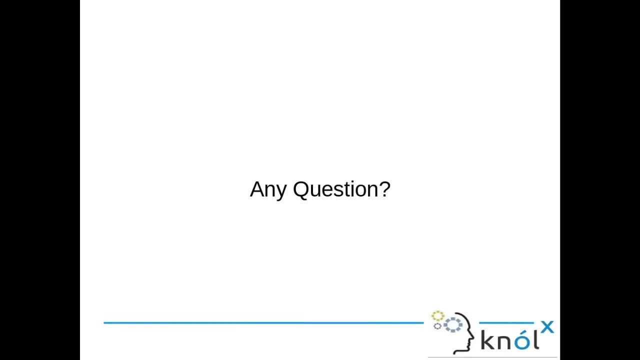 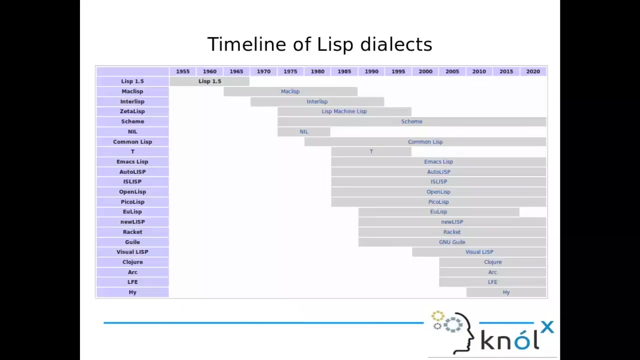 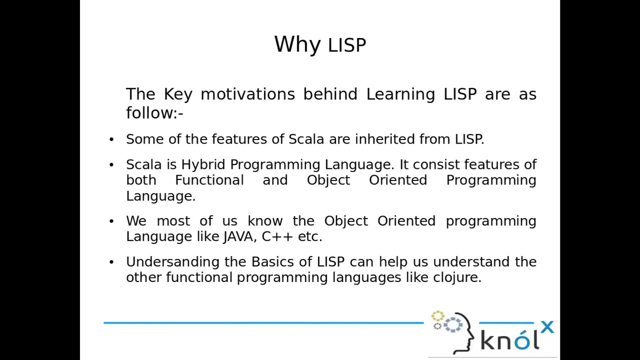 We can accept the argument and at the same time we can also return the high order function. So there are much more complex features that are present in the list that I will cover in the next knowledge. One of the main reason is that, as I shown in the first slide, some of the features that are present in Scala into the functional approach way are inherited indirectly from the list programming. 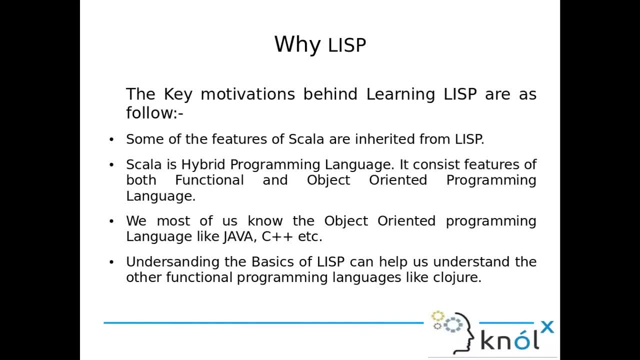 So basically, to have what we have. our mind is. our mind set is basically focused on the object oriented programming way, Because we know everything is an object when we compute everything in that form. But from functional approach things can slightly change, So that's why we are learning this. 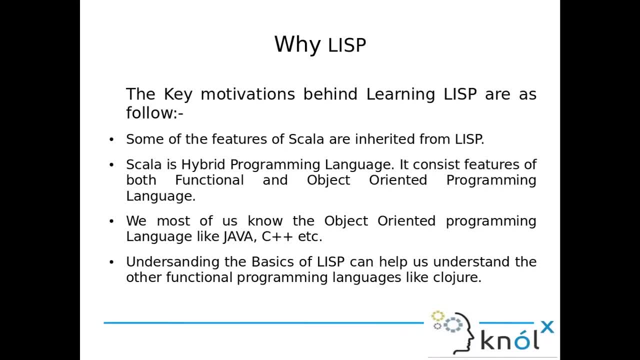 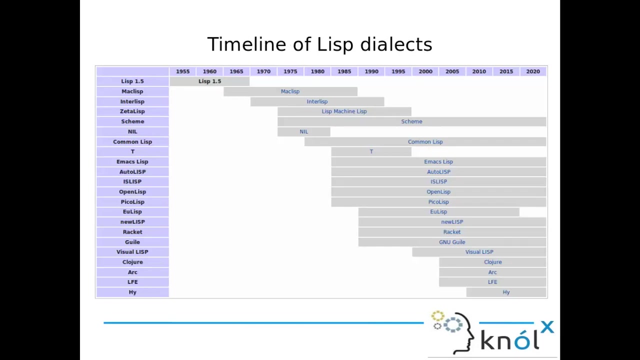 Yes, Yes, Yes, You can see here the closer is actually inherited, the list is inherited inside the closer, And there are some more functional programming that I can write that are actually still not popular till now, But closer is quite popular right now. 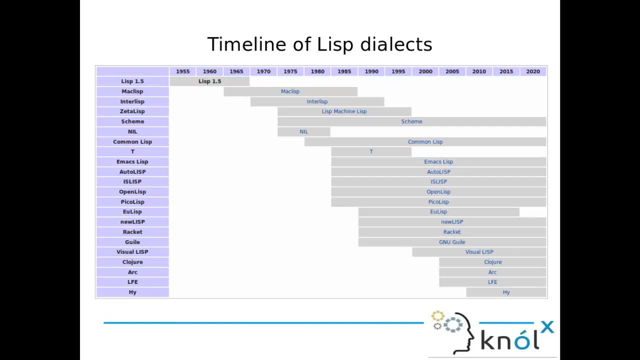 Yes, but for example, most of us know Java before learning to the Scala. So that's why our approach is slightly same as the object oriented way That everything should be in object. 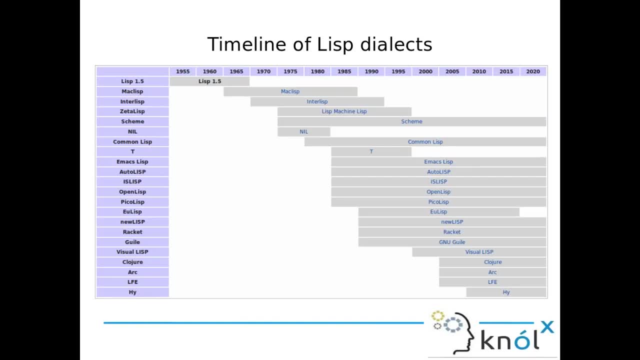 We used to use the where initially in the Java, we will learn how these values are actually problem inside that? no, actually it is not, but it is actually help us enhancing the more we can use the more feature of the Scala in more functional approach we can take it. and I think I need to start with, even if we know 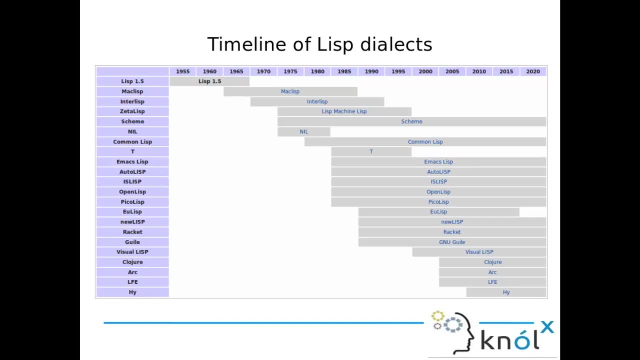 that it is not very much complicated. so it is very difficult and, if I can evolve, so once there was a project and it might ask us to make a book as a website. it is a very simple book, so it is better and it is a piece of computer program. so, and I think that to be